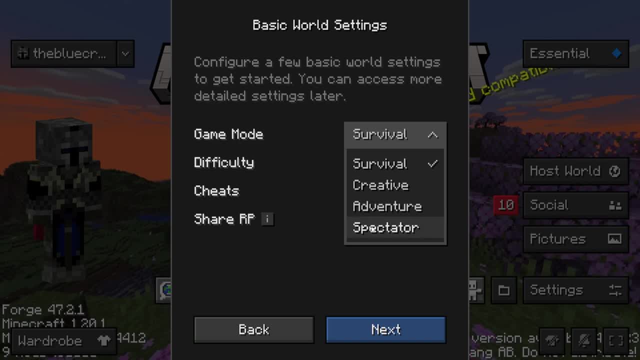 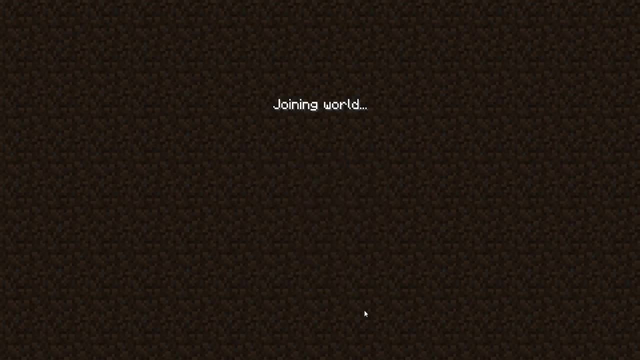 Imagine a world where you can play together without a server, for free. With Essential, you and your friends can team up for adventures without pesky fees and connections. that would be if you actually paid for a server. The chat system is your personal messenger, pigeon. 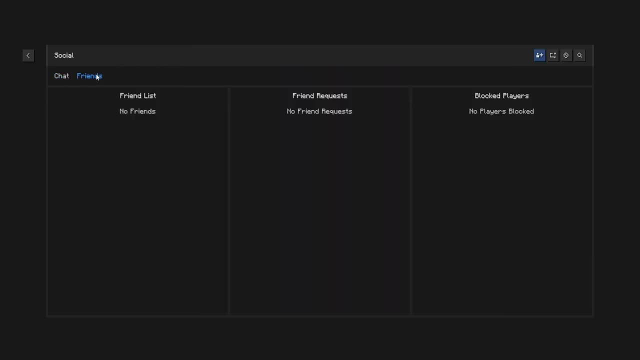 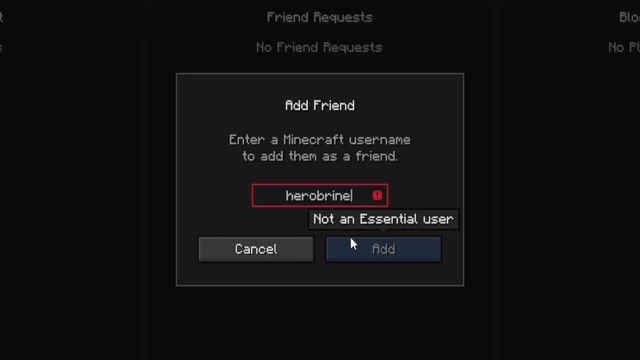 Chat plan, joke around with your friends across different worlds and servers to organise your alliances in groups, whilst you mine and build to your heart's content. And why limit your creative expression to just using blocks? With Essential's wardrobe feature, you can get to dress up your character in a one-of-a-kind set of outfits. 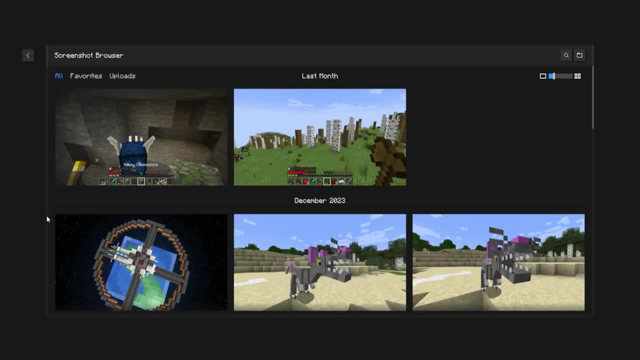 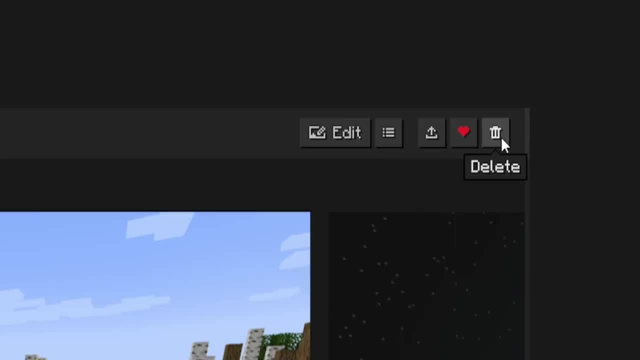 to let your avatar mirror your style. Ever wished you could capture your moments and share them without a break. in immersion Essential lets you capture, edit and share those victory moments or that perfect sunset on multiplayer, right from within the game, with its screenshot tool. 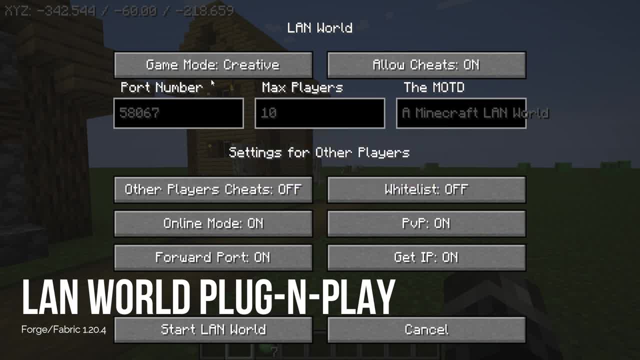 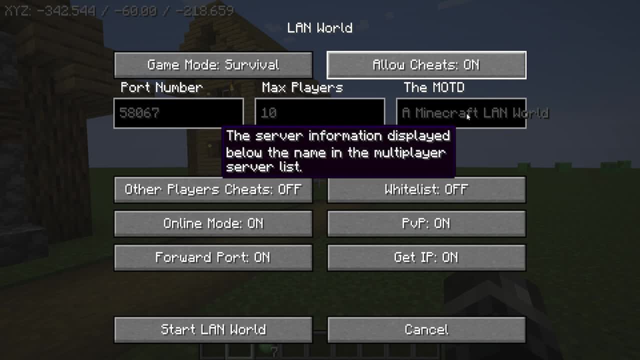 Before LAN World. plug-and-play hosting a server was like defusing a creeper bomb: Tricky, confusing and probably likely to end in disaster. and you have to read so many tutorials. You had to mess with port forwarding and player permissions and modes. 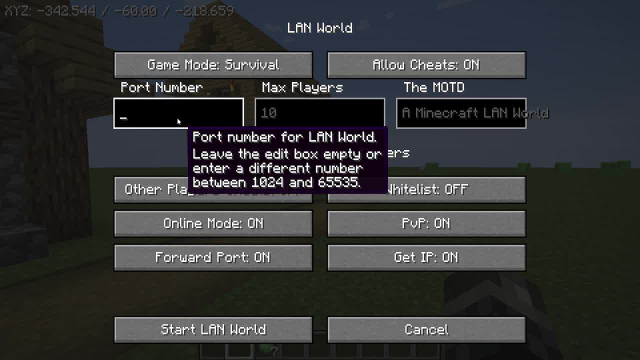 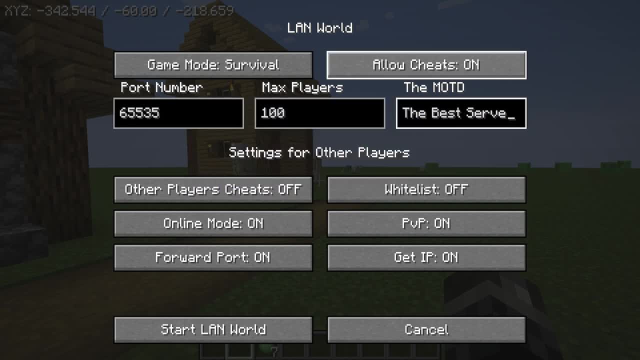 but with this mod you can tweak the port number of your LAN World and map it out to your public network, all with a simple flip of a switch. You can turn on PvP if you so wish. set the message of the day of the server. 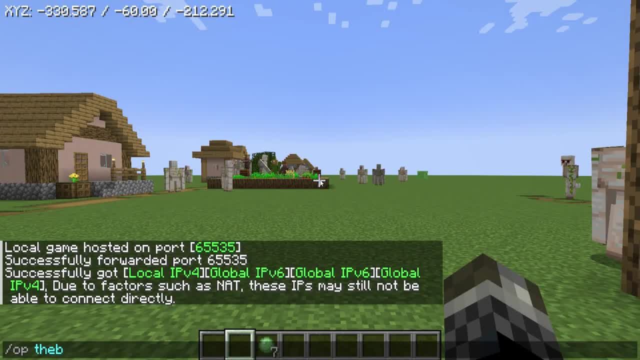 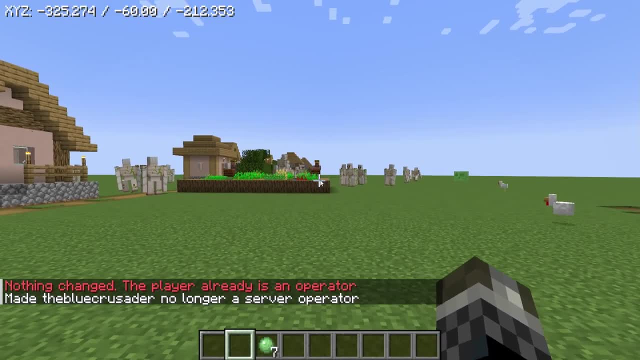 control permissions of the players with a simple OP and DOP command, and even use a whitelist to control who plays. You can join your world. The cherry on top: all of your settings are saved, automatically loaded the next time you log in. The friends list feature is a gateway to new friendships. 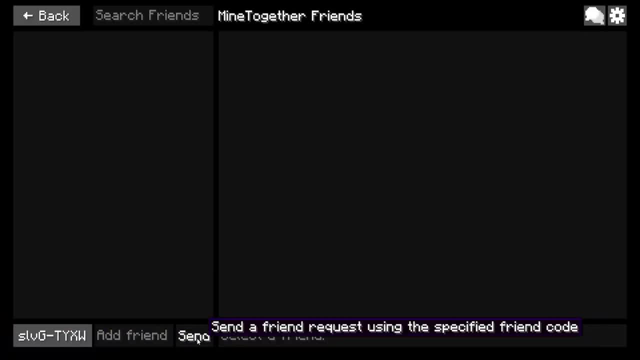 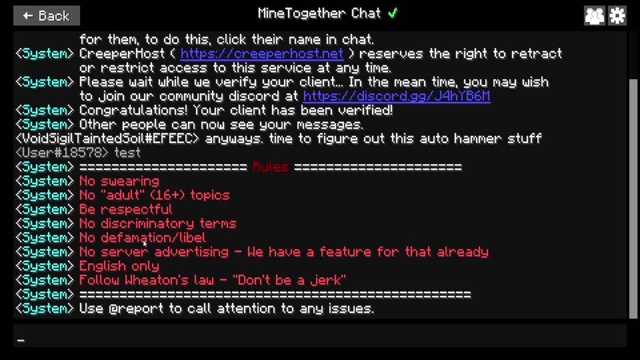 shared victories and laughter. It's the tool that lets you reach out across the server divide, forging alliances. But what's that without the communication? The mod also brings global chat and group chat features, breaking barriers and opening new channels for discussion and strategic planning. 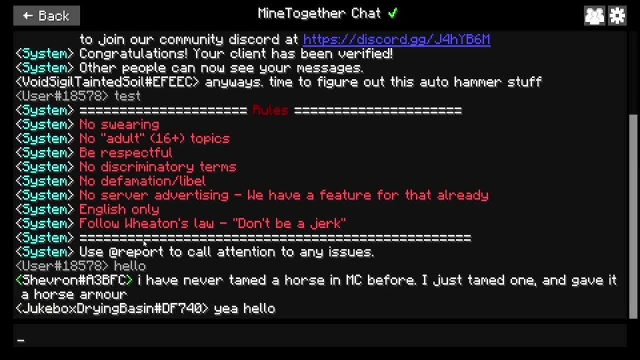 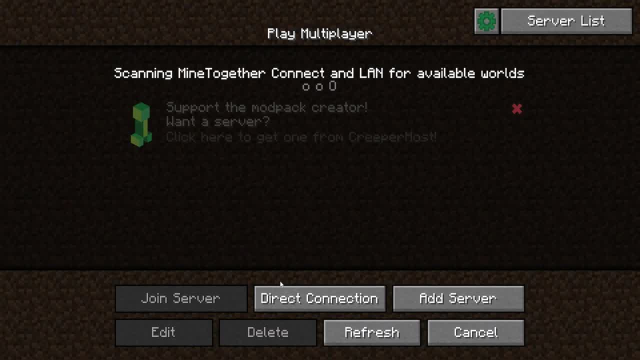 Got a new redstone idea, Share it with the world. Found a new rare biome. Shout it out in the group chat. But for the more secret conversations, the messages feature steps in. And as we navigate through our options, the server list is our compass. 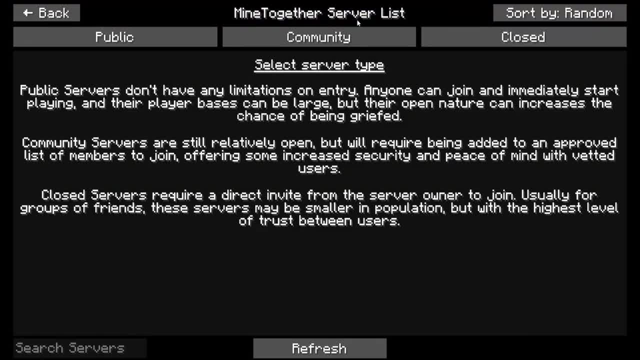 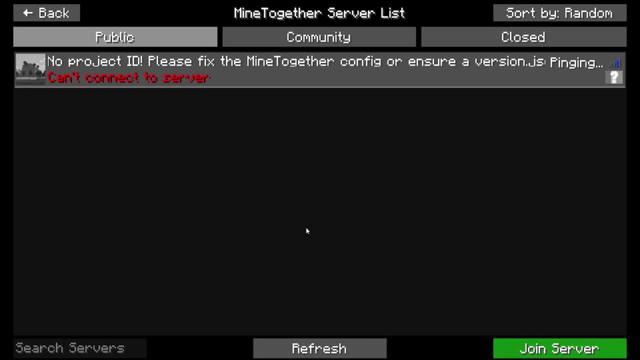 With the world pre-generation feature, you no longer have to arrive in a half-loaded world. The mod also brings private minigames, personalized arenas to compete and show off your skills. With the server invites feature, you can invite your friends over for a session of building or survival. 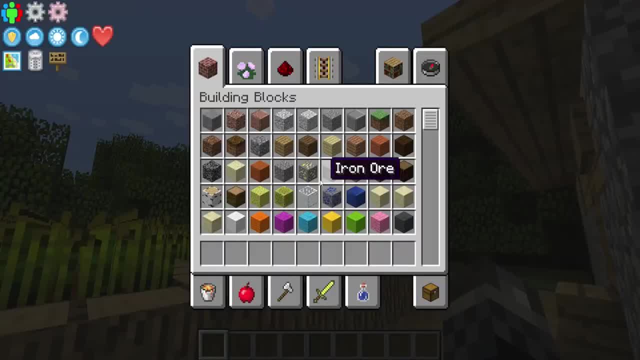 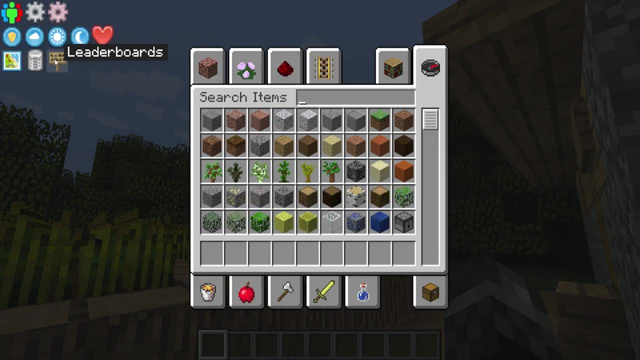 FTB Utilities is the Swiss army knife of mods with Chunk, claiming your land and constructions are safe. No unwelcome visitors will even think of touching it. You're deep in exploration and, as the sun sets, the nearest safe haven is a world away. 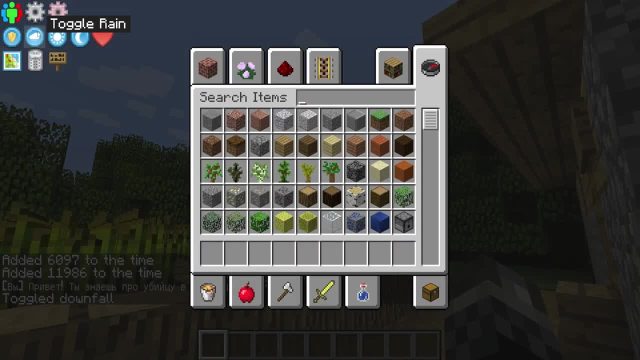 Wouldn't it be great to teleport to safety in a second. This is where the mods TPA, or teleportation, shines. With just a command, you'll have yourself back at home, away from monsters. The auto shutdown feature ensures the game runs optimally at all times. 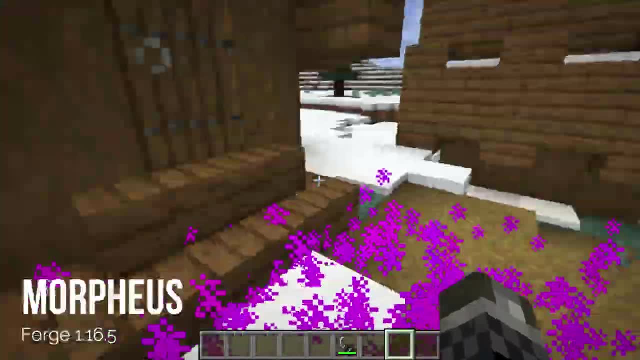 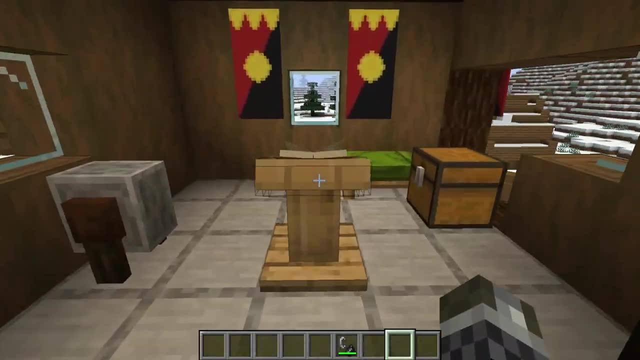 without draining your system resources. Morpheus is a server only mod. Think of it like a sleep democracy. It introduces an ingenious sleep voting system where players can collectively decide amongst themselves when to fast forward to morning time. When a player decides to sleep. 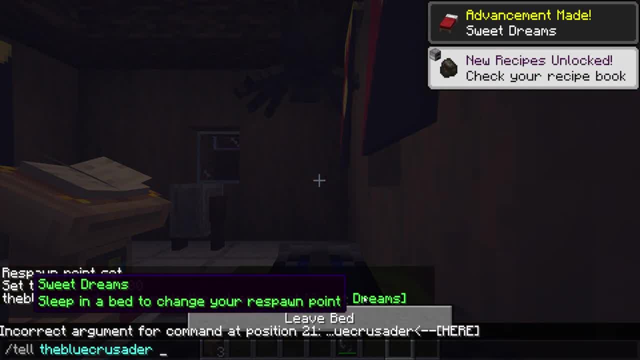 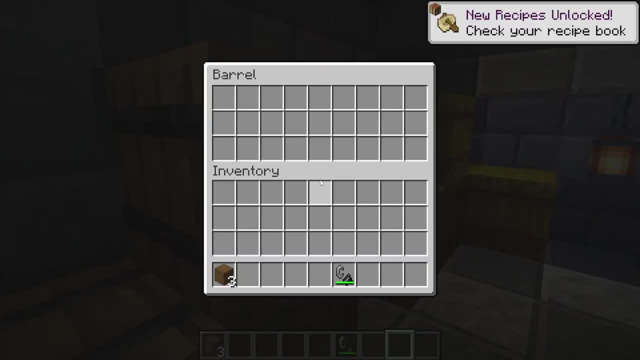 a notification is sent out to all players within that same dimension, allowing everyone to coordinate on vote: whether to turn night to day. The ratio of players required to initiate the sequence can be customized. By default, it's set to 50% to make things fair, but it can be tweaked. 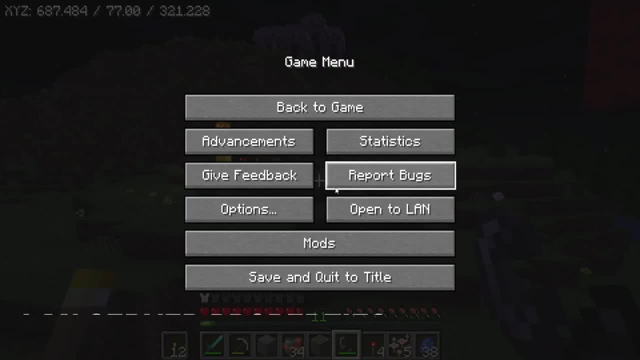 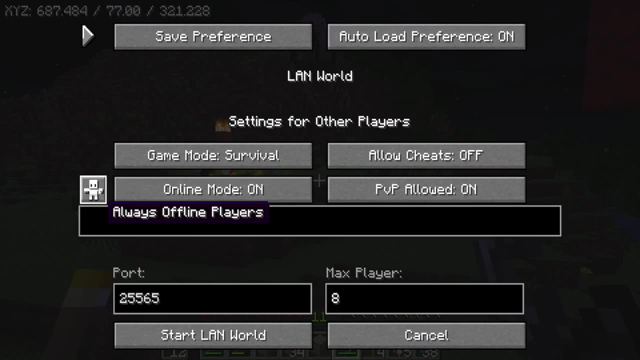 You can also turn off sleep alerts, allowing you to roam undisturbed. Imagine setting up a land game on a specific port of your choosing. You can also toggle the online mode to choose whether you want to be online or offline. You can enable or disable PVP. 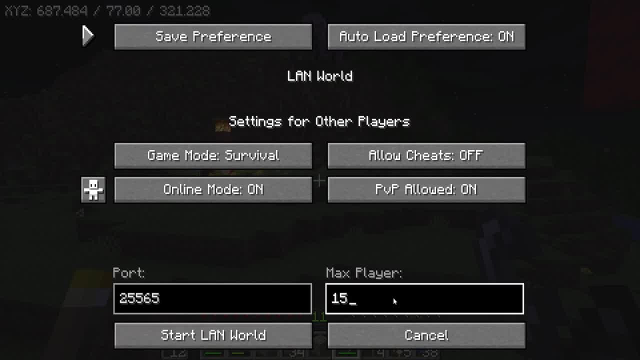 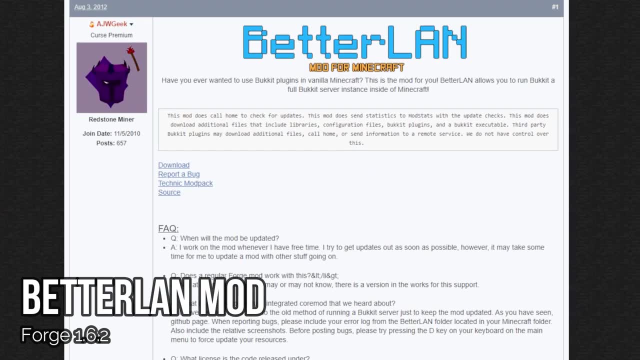 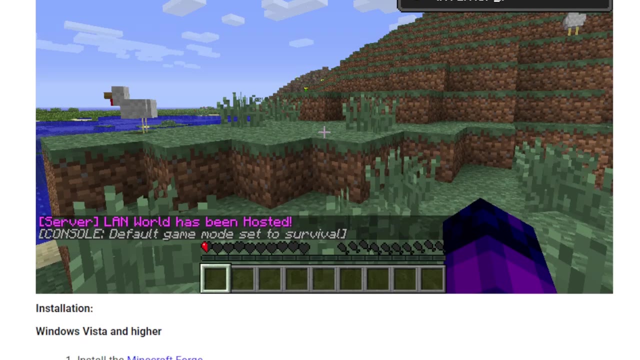 Set a maximum player count and after version 1.19, you can prioritize the UUID from Microsoft or Mojang accounts wherever possible to prevent losing items during mode switches. Ever wish to run bucket plugins over LAN or even share a tech kit server? With this mod, you can seamlessly integrate unmodded clients and even Hamachi. 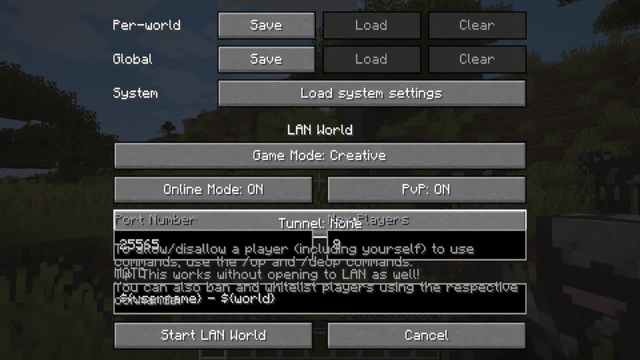 This mod allows you to customize a wealth of features, from online modes, PVP settings, max players, right down to your MOTD. You get to call the shots. What's more, if you're in the middle of the game and you wish, 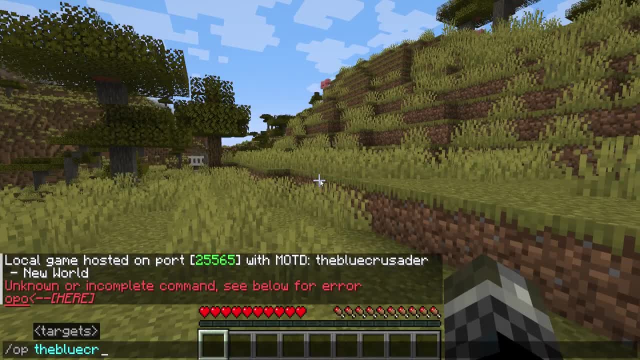 to tweak some settings. you don't even need to restart. You can quickly use the OP and DOP commands to grant some power And if you're tired of enabling cheats, each time that you want to bend the rules a little, these commands will save you. 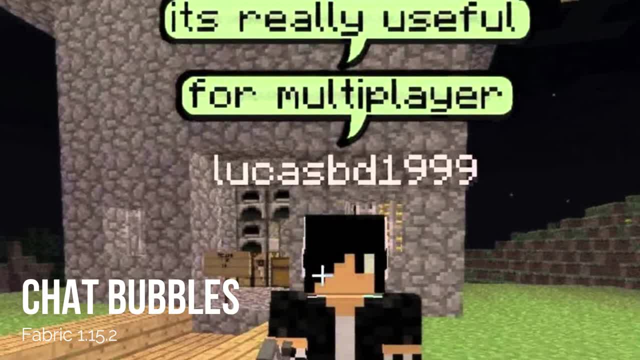 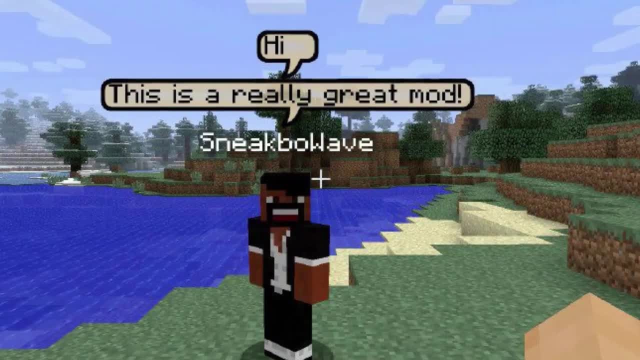 This is a simple mod that adds messages that display above players heads in the form of a chat bubble, just like in many MMORPG games like RuneScape or Virtual Worlds of the early 2000s. This is a small quality of life mod. 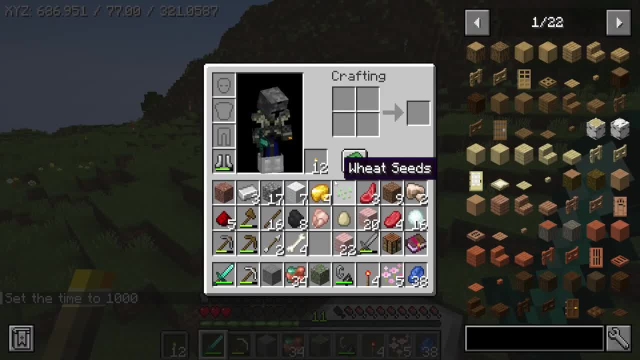 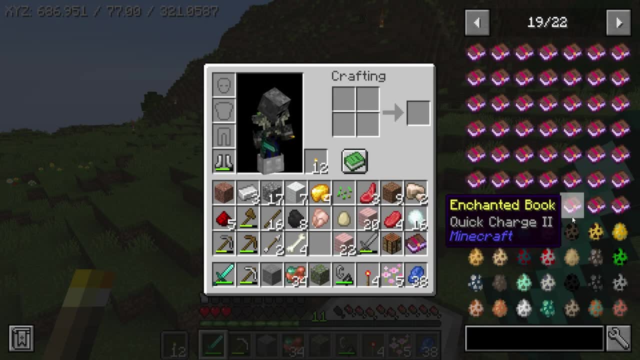 but it looks attractive and it's a nice feature to add to Minecraft multiplayer. Everyone's favorite recipe viewer, Just Enough Items, is a client side mod, but it's one of the essential mods everyone needs And it's more powerful when run on the server side.